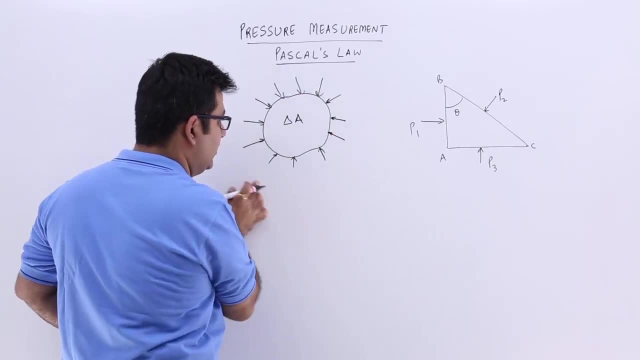 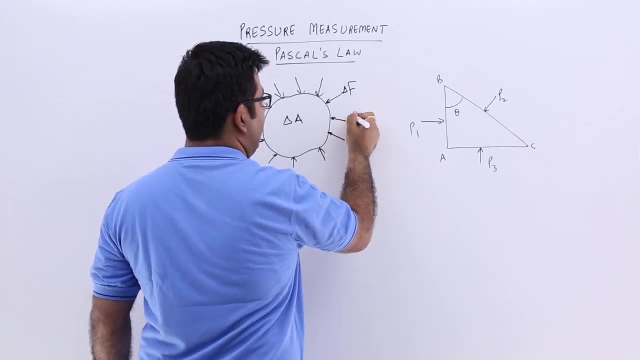 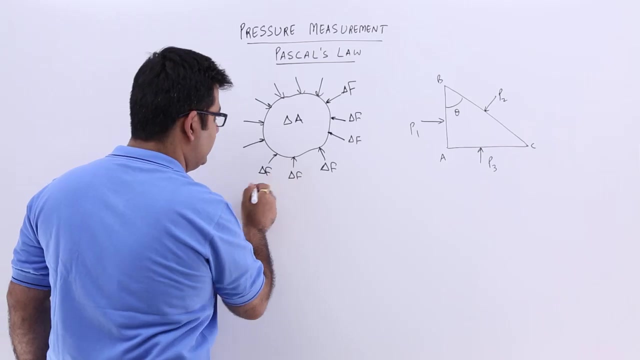 Okay, and always remember this, This force which is being exerted from all the sides is always perpendicular. So this, Let us say, is delta F on all sides. All these small elementary force elements, They sum up to create the entire force on this element. 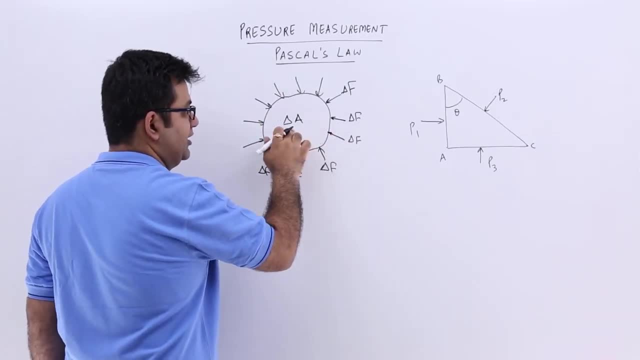 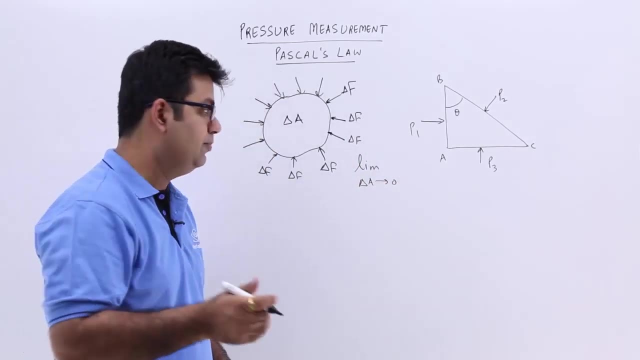 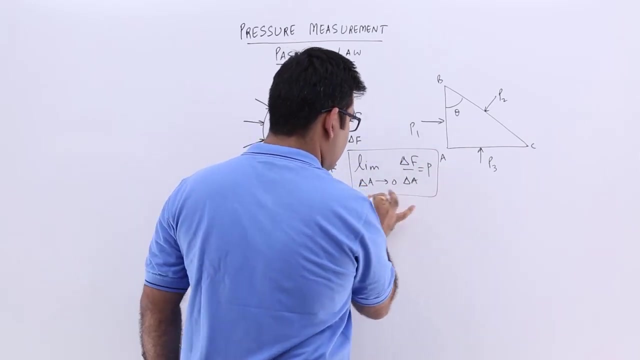 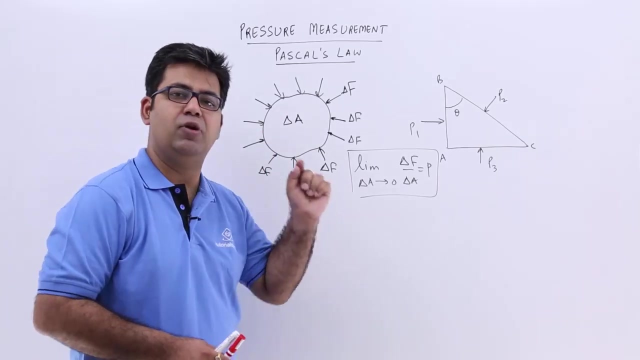 So, if you take the ratio between this force and this area- And let us say the area is so small that it almost tends to zero, So delta F upon delta A, This is known as The pressure on this fluid element. Okay, now I told you that the force has to be always perpendicular to this fluid area. 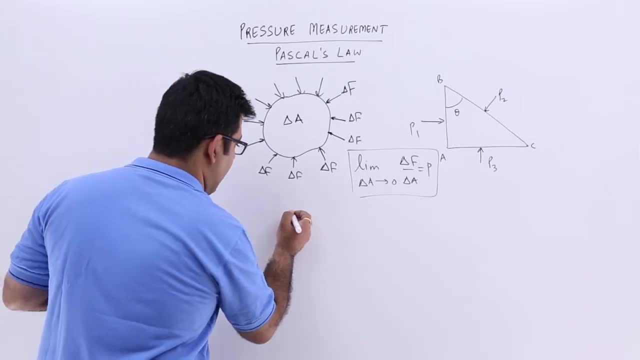 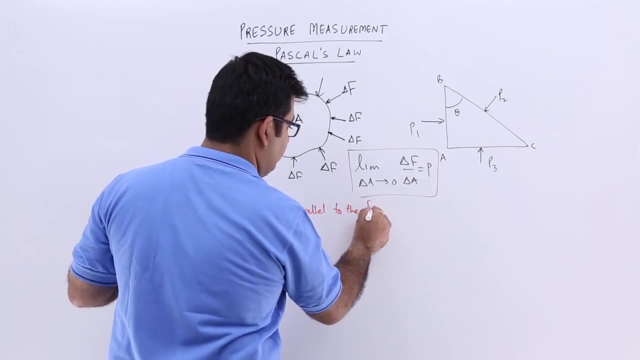 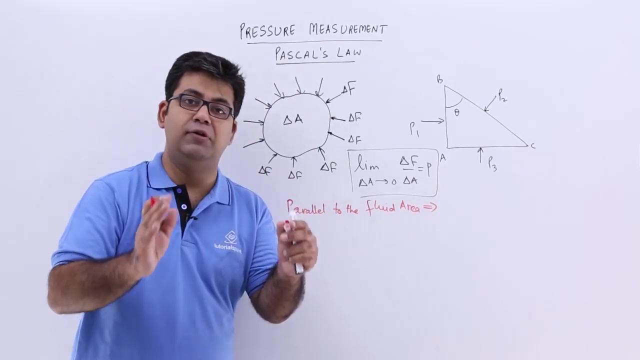 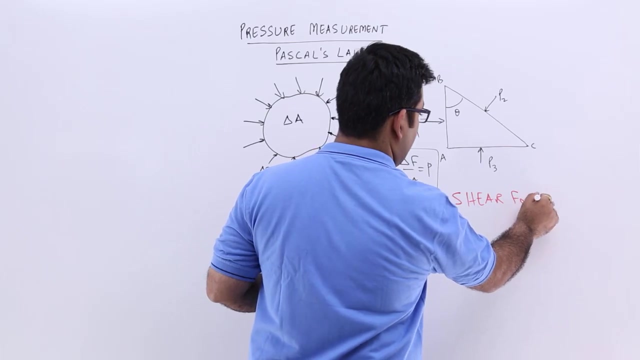 And there can be other force also, There can be a force which is parallel, Which is parallel to the fluid area, Which is parallel to the fluid area, And this force, which is Parallel to the fluid area, is called the shear force, Is called the shear force. 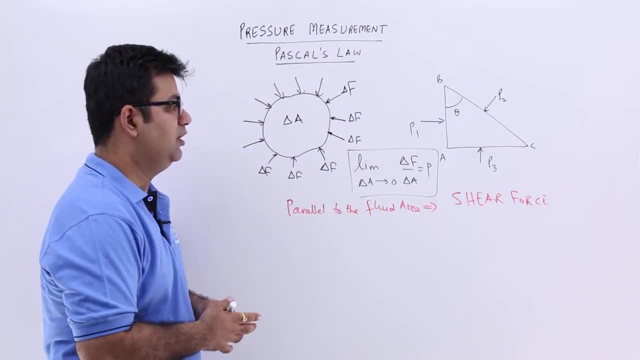 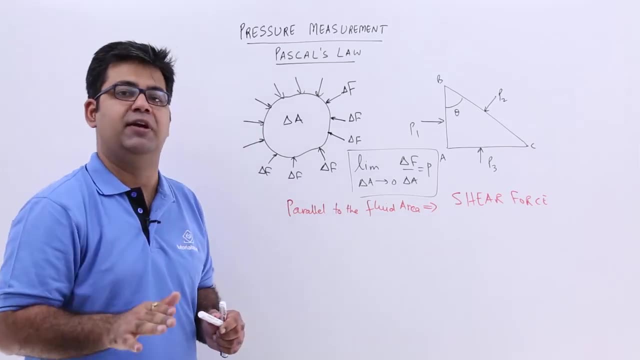 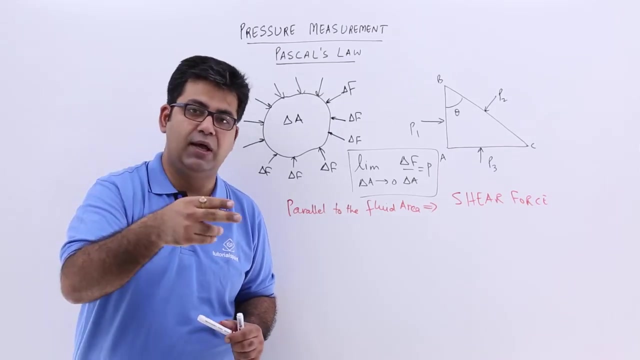 Now, very big difference is there When we talk about the shear force And when we talk about the pressure force. Okay, Shear force, or the shearing effect, Comes into picture only when your fluid is in motion, That is, two adjacent layers of fluid are in relative motion with each other. 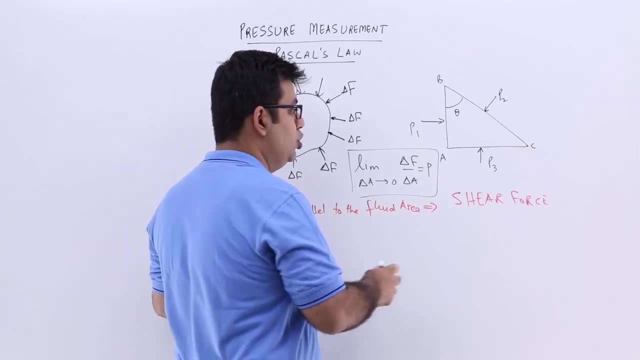 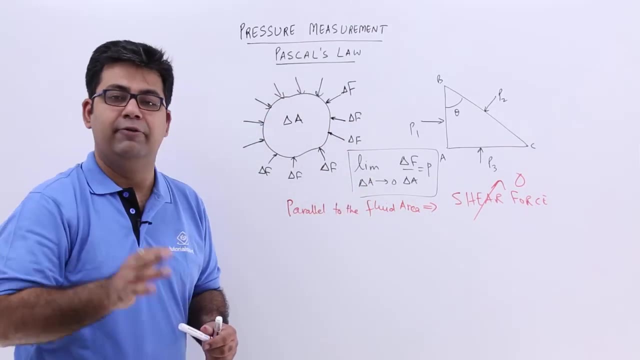 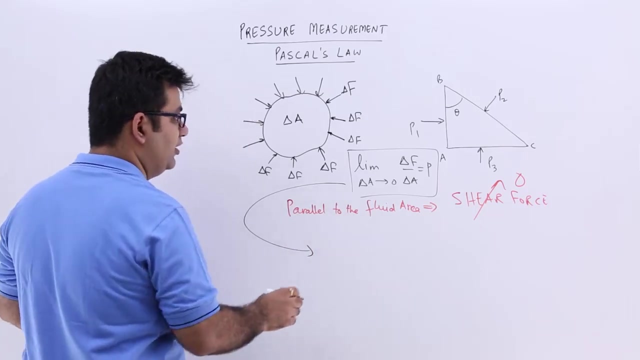 Okay, So if your fluid is at rest, Then there is no question of shear force arising. So there will be no component of this force Which will be parallel to the fluid area. So there will be no shear force. Okay, So this means that we are more concerned with the pressure force. 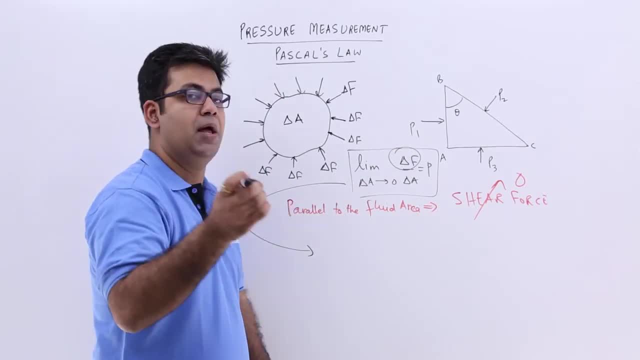 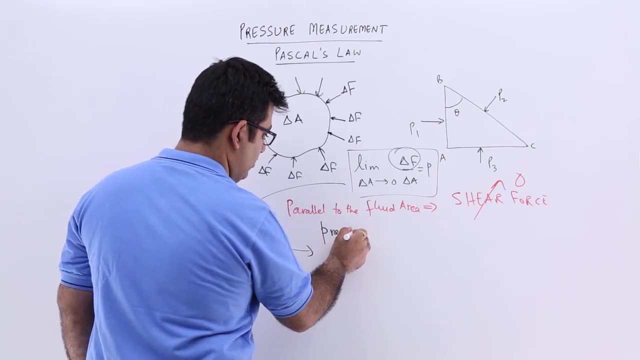 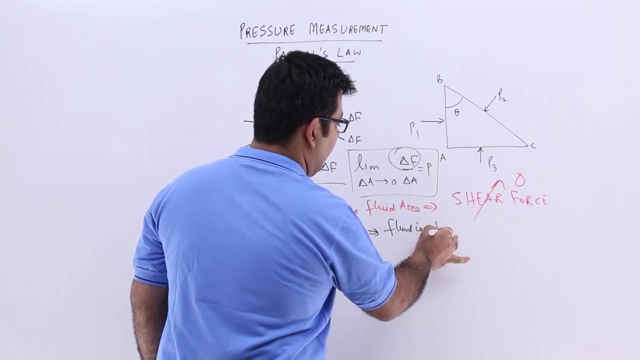 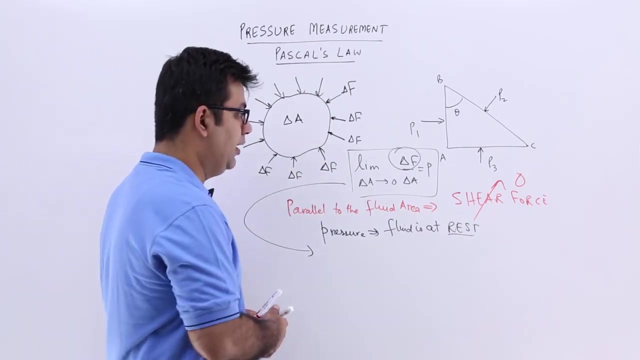 Or that component of force which is perpendicular to this fluid area. Okay, So we consider pressure. We consider pressure When The fluid is At rest, That is, When the fluid is static, It has no motion in it. Alright, 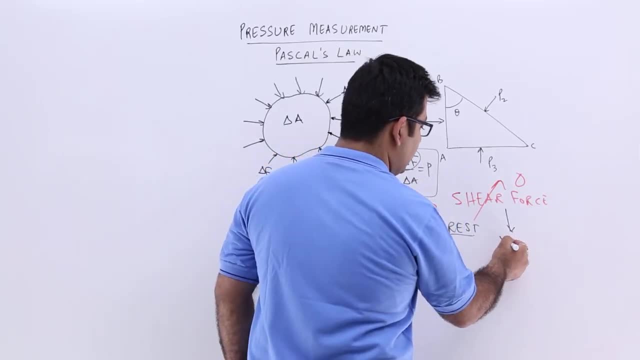 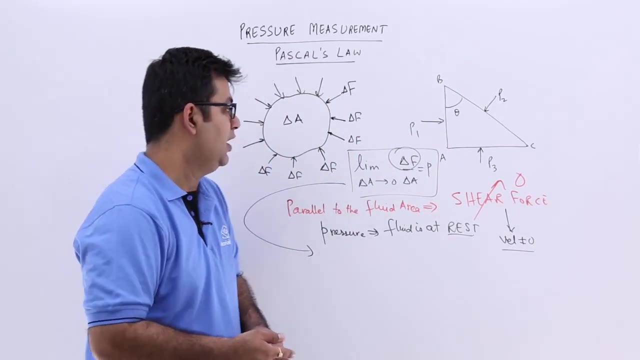 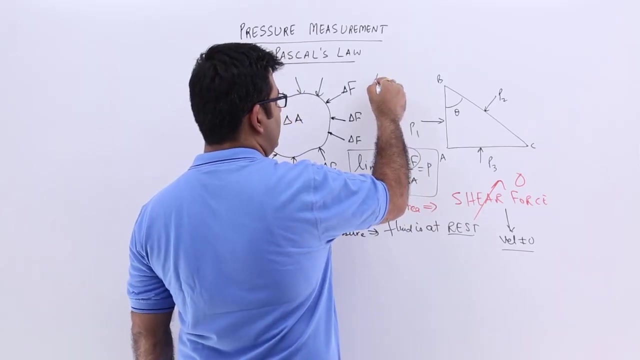 And shear force is considered When there is some velocity, So the velocity should not be zero. Okay, That is, the fluid is in motion. Now we have defined pressure. Now, what is the units of pressure? The units of pressure, So the unit of force is neutral. 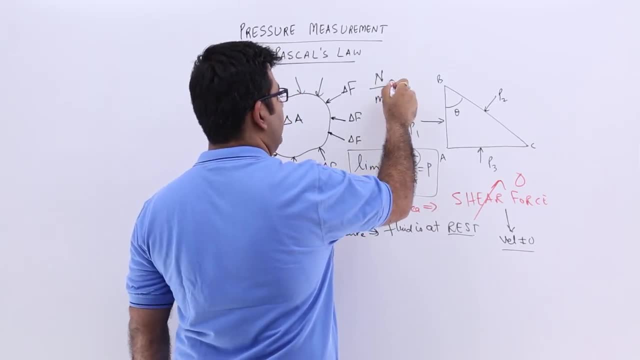 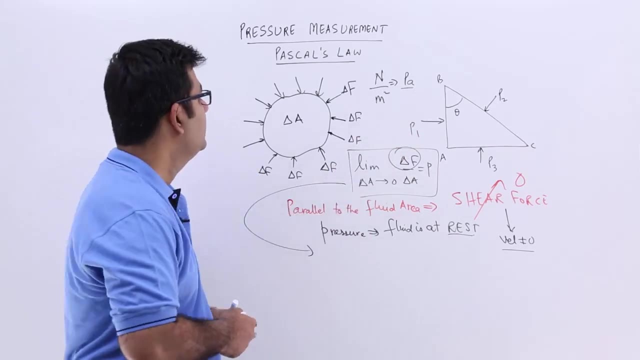 Newton's, And the units of area would be meter square. So this would be Newton per meter square, or Pascal. Now, with the units of The pressure as Pascal's, Let's come to a law Which is the Pascal's law For fluids. 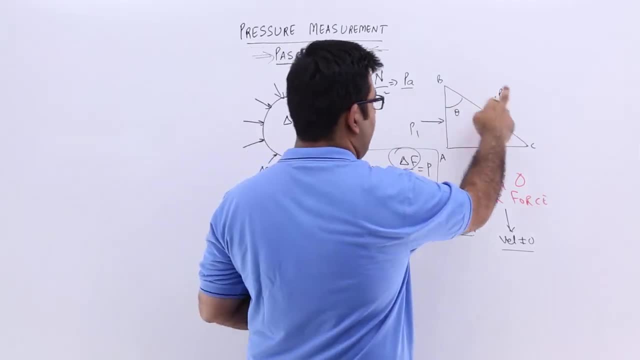 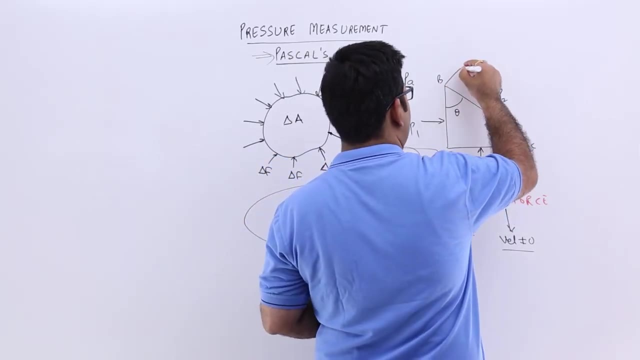 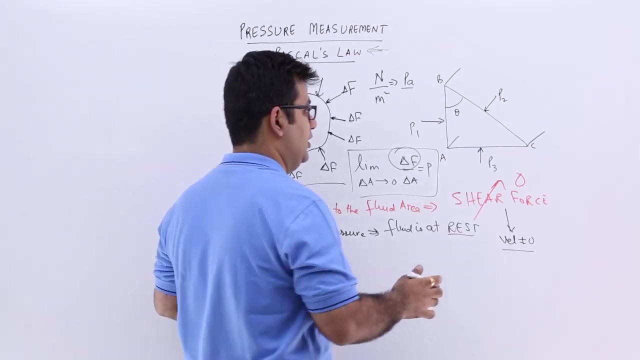 To understand Pascal's law. Let's consider This element of a fluid. Okay, This is a wedge Element. It has some thickness to it, And let us say that thickness Is one, So the thickness of this wedge element is one. 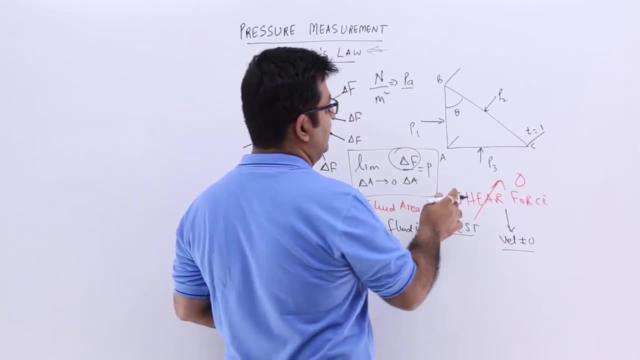 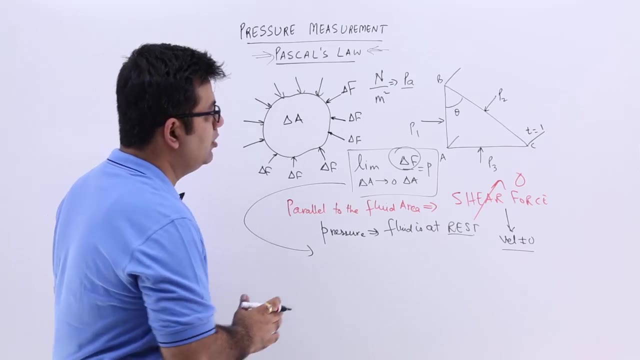 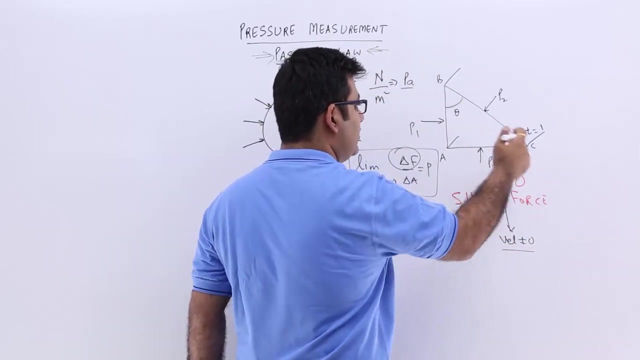 Whatever, the units are Okay, And it has an angle theta in it And you have three sides: AB, BC and CA. Okay, and on side AB You have a pressure P1. And on side AC You have pressure P3. 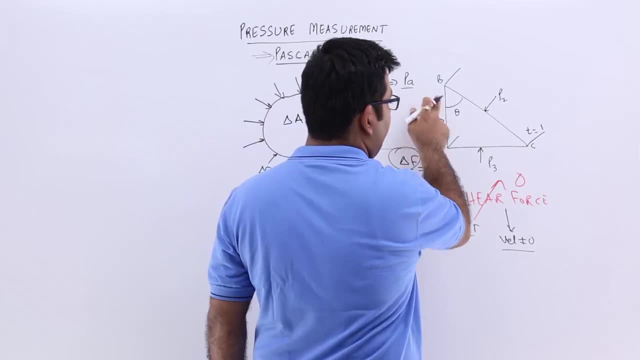 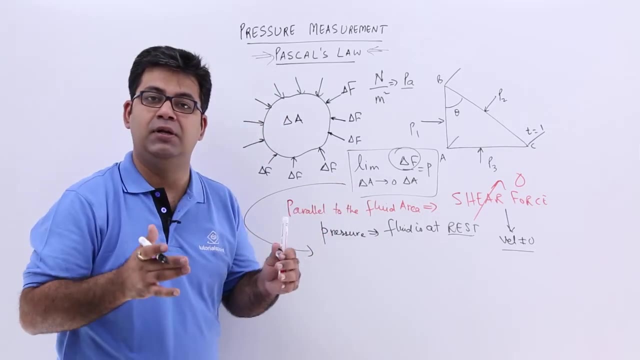 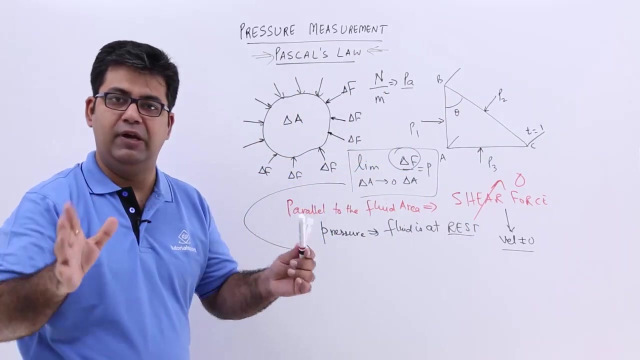 And on this inclined side, At theta to the vertical, You have a pressure P2.. Okay, Let's resolve these pressures In horizontal and vertical Direction. So let us say this entire Wedge fluid element is in equilibrium. Okay, so the pressure force. 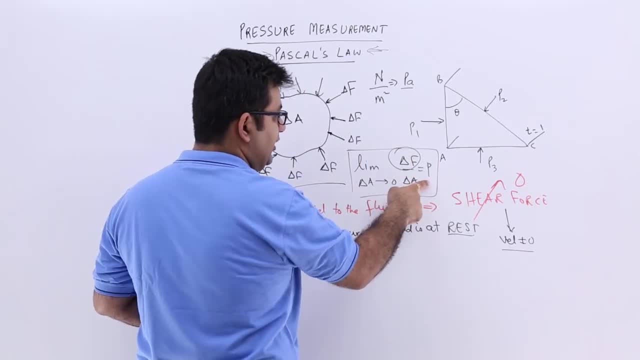 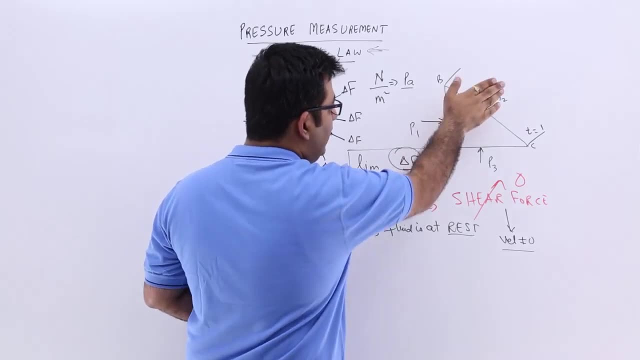 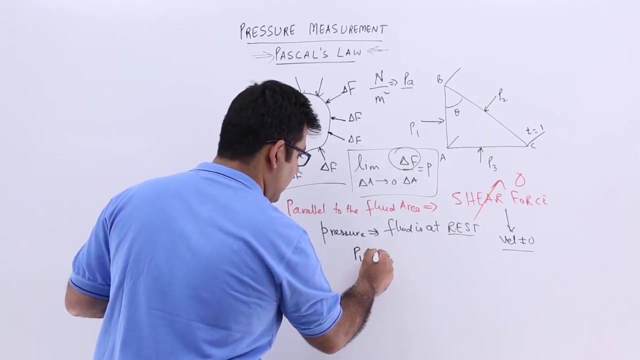 On the side. AB Would be pressure into area, So pressure force is Pressure into area, So pressure is P1. Area would be AB into the length Or the thickness of the wedge, So it will have P1. Into AB, into one. 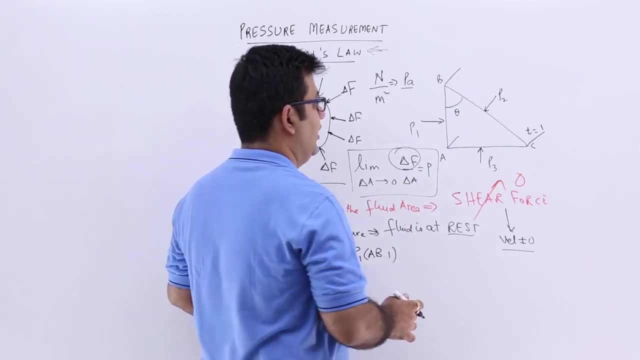 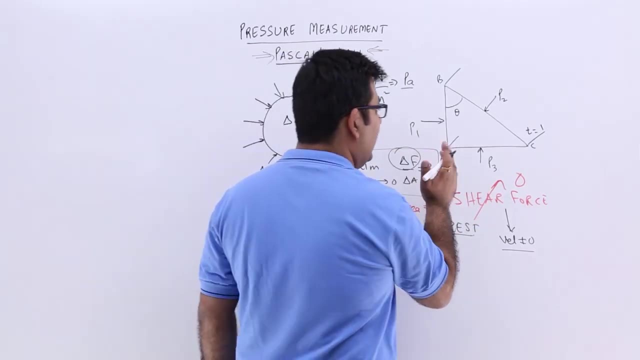 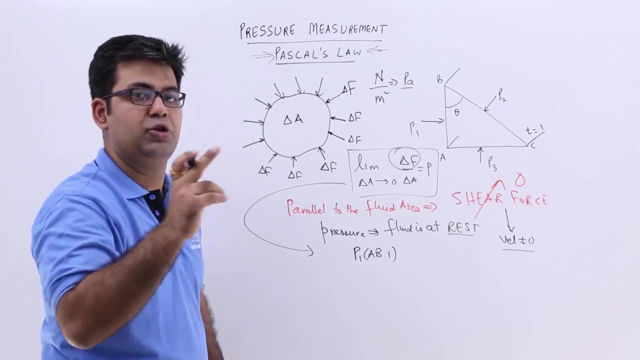 Because the thickness of the wedge is one. Okay, Now, if you look at this pressure, It will have no horizontal Pressure force element Because it is entirely vertical. But if you come to this inclined Pressure component, It will have one vertical and one horizontal. 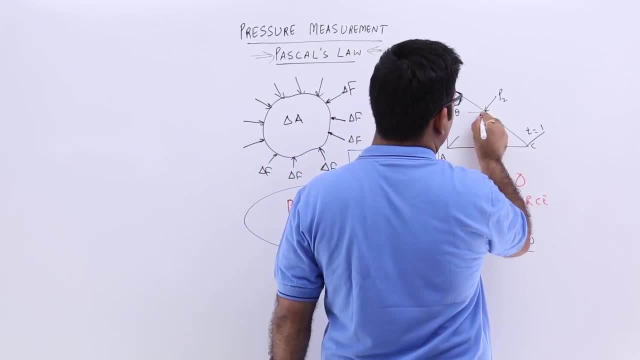 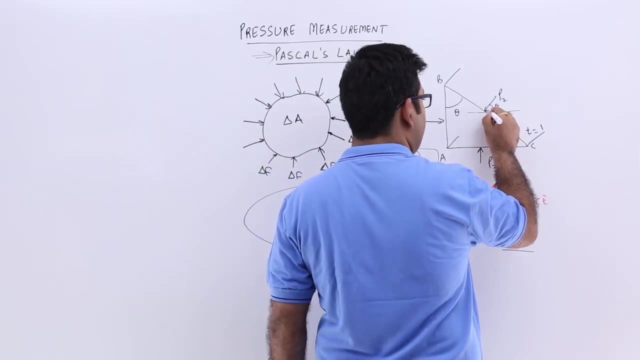 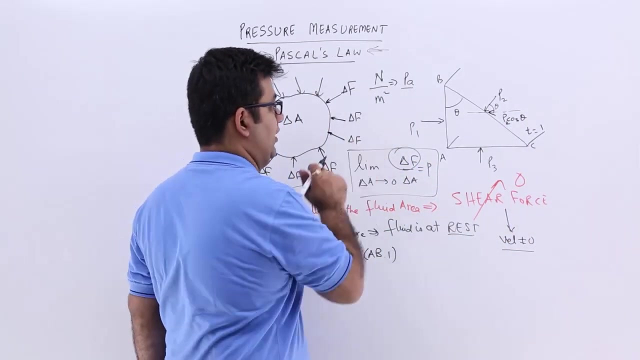 Pressure force component. So if you draw a line like this, With simple geometry, This angle will be theta. So you will have Pressure component which will be P cos theta Or P2 cos theta In this direction Which is opposite to P1.. 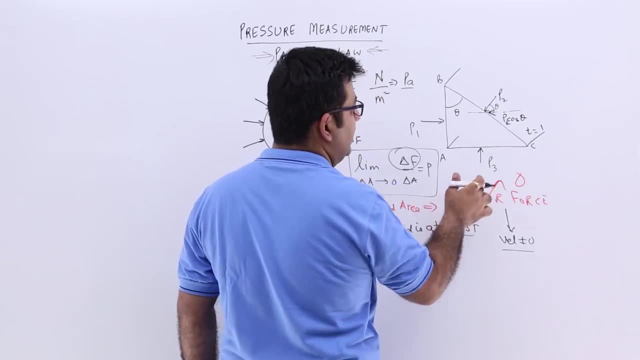 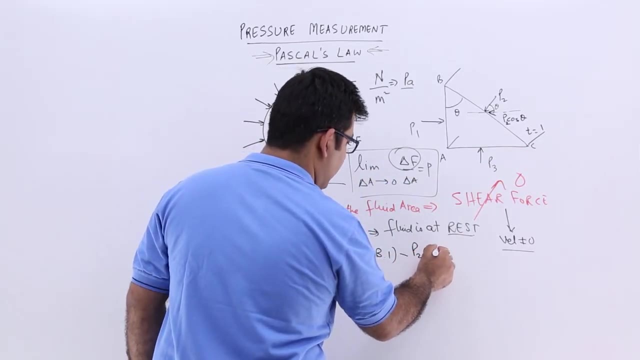 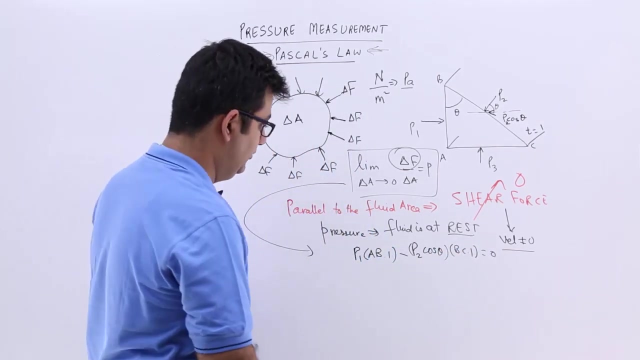 Okay, so the pressure? The pressure would be P2 cos theta Into BC, So minus P2 cos theta Into BC Into one. Alright, Now let us Take the geometry into consideration, Or I would say right angle triangle. 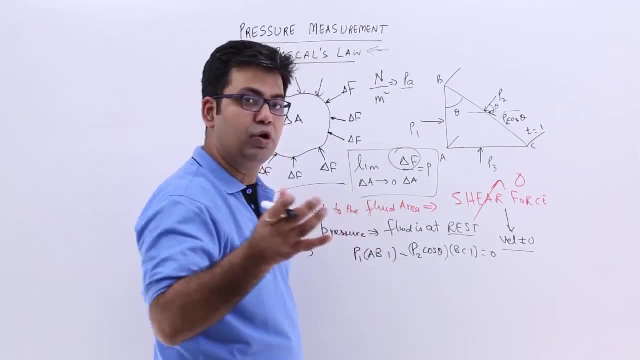 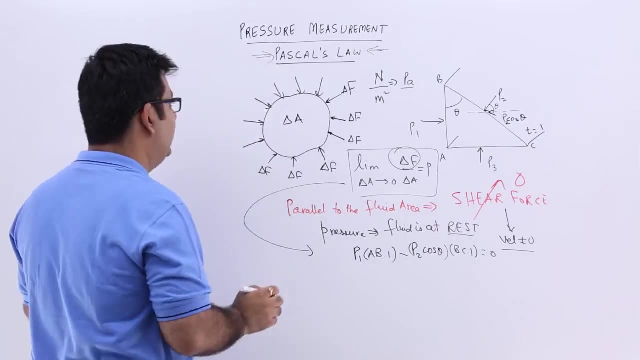 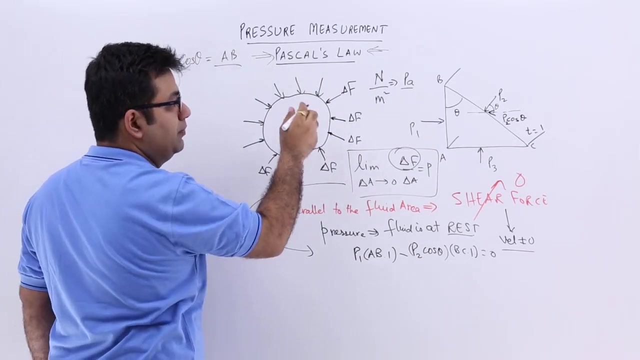 Trigonometry. Okay, If you find out cos theta, Cos theta would be base, That is AB upon hypotenuse, Which is BC. So cos theta? If I write down over here, Cos theta is equal to AB Upon BC. 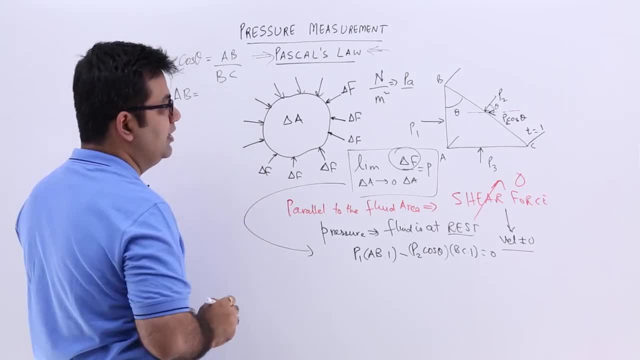 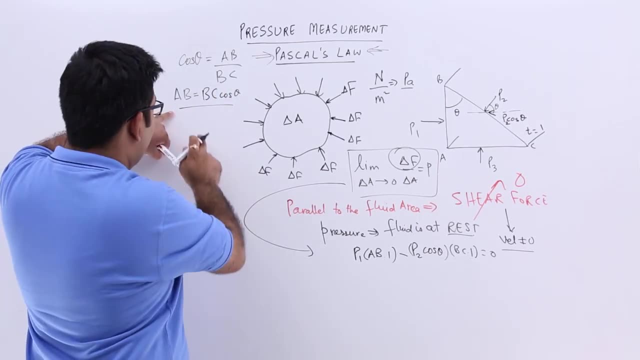 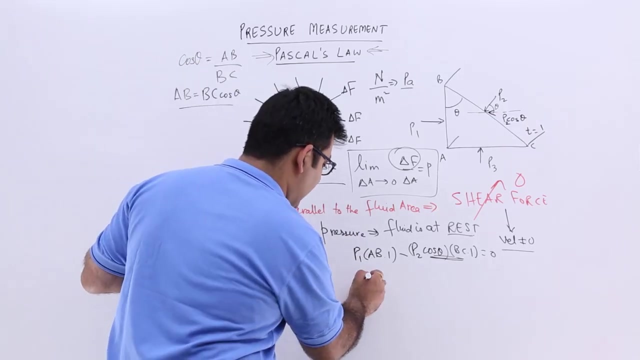 So from here I can say That AB is equal to BC cos theta, AB is equal to BC cos theta. So from this Value I can substitute BC cos theta As AB. So I can say that P1. Into AB. 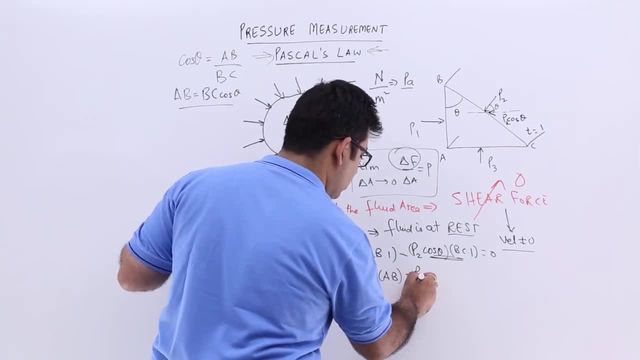 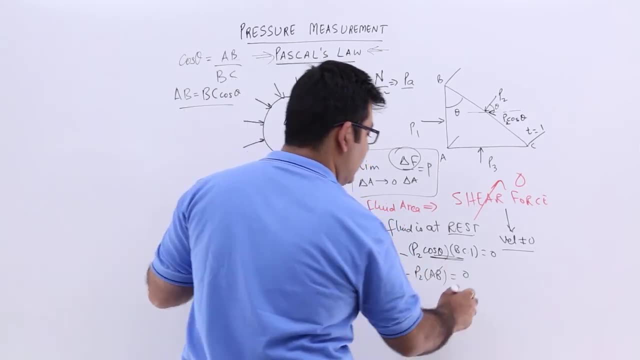 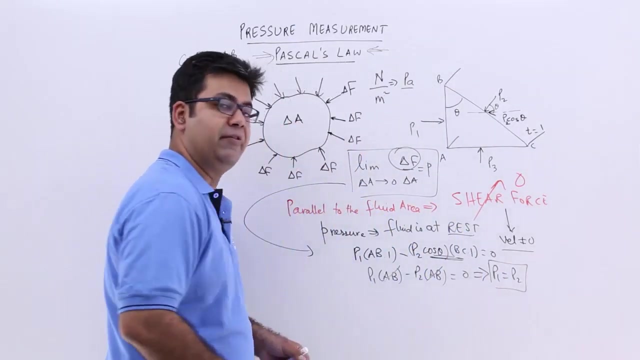 Minus P2.. Into AB, Because that is equal to BC, cos theta Equal to 0.. You can strike off AB and AB And this gives you A value which says P1. Is equal to P2.. Now, after P1 is equal to P2.. 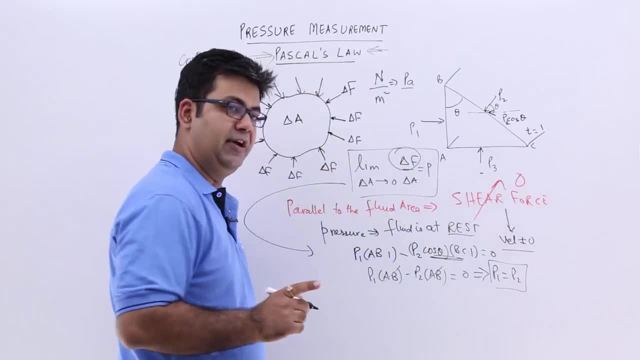 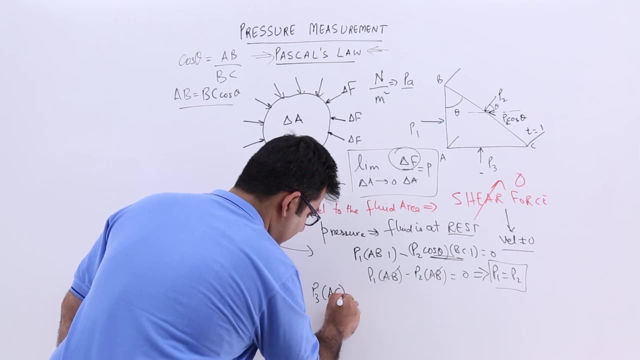 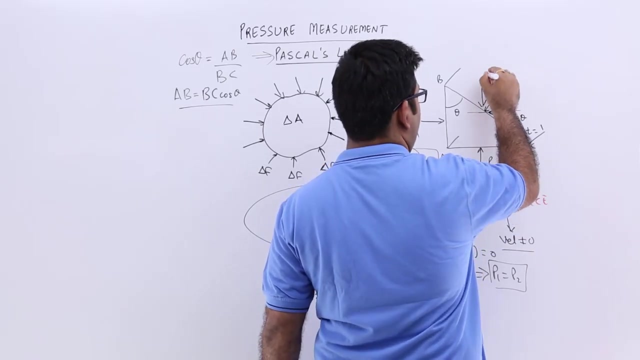 Let us consider the Vertical component. So the vertical component will be P3. Into AC into 1.. So we will have P3. Into AC into 1., That is, vertically upwards, And P2. Will have a vertically downwards component. 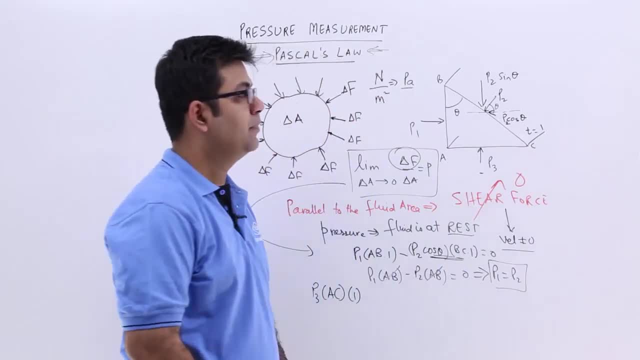 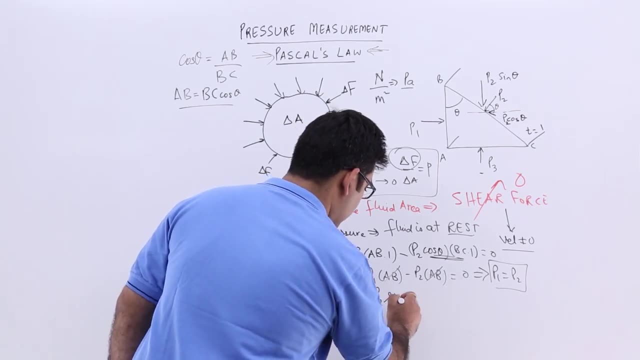 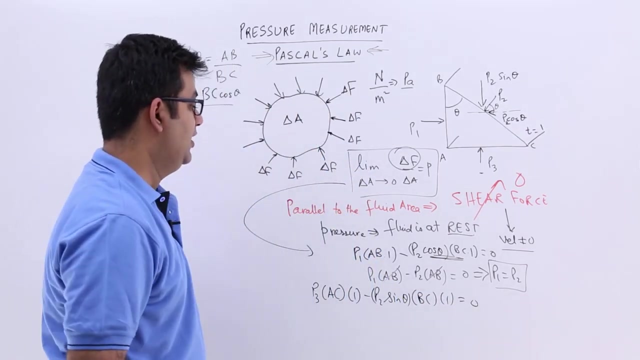 Which will be P2. Into sin theta And that will be P2 sin theta Into BC. So minus P2. Sin theta Into BC Into 1. Is equal to 0.. Now again, I will use the right angle triangle. 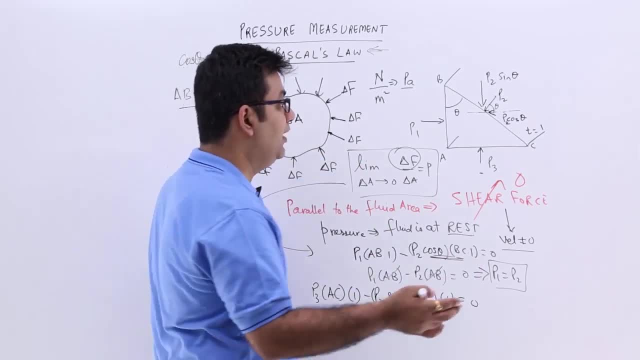 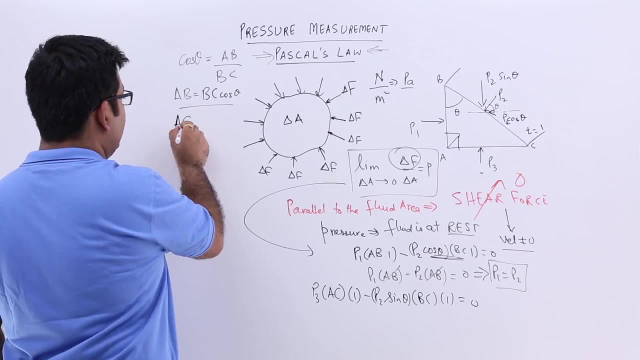 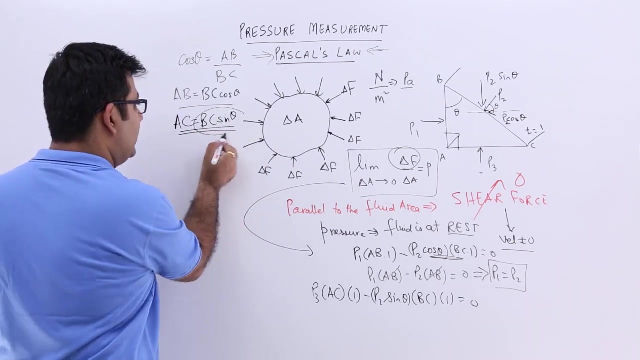 And find out sin theta from there. So sin theta would be Perpendicular AC Upon BC. So I can say That AC Is equal to BC Into sin theta. So I will substitute BC sin theta Over here As AC.